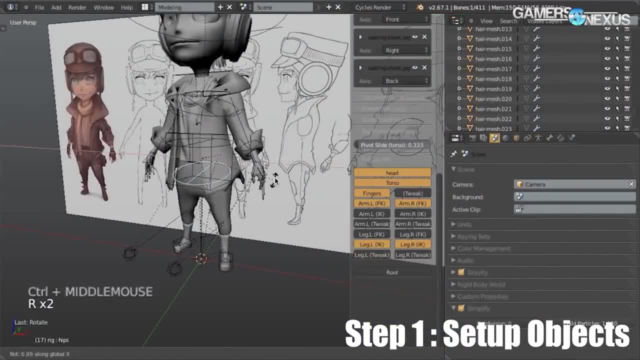 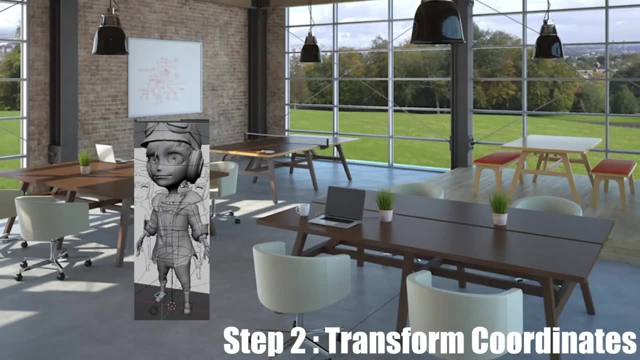 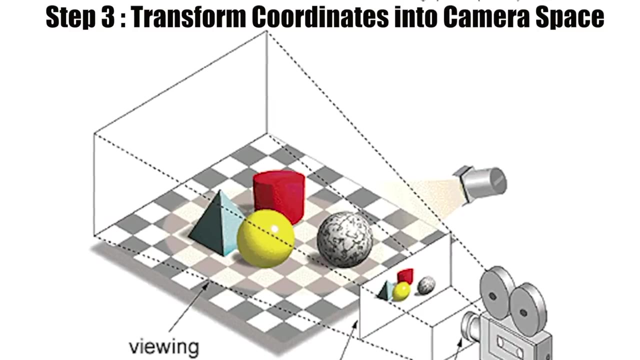 the exact coordinates of every corner, of every triangle. Coordinate systems need an origin, and in a models file it's just an arbitrary place. But to place the model in the scene all the vertex coordinates need to be transformed so that the origin is now a place in the scene. Once the objects are placed in the scene, 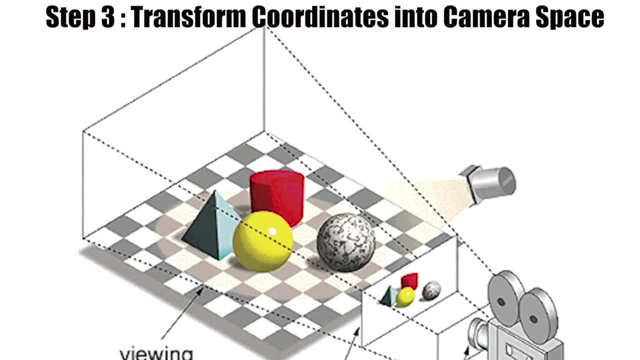 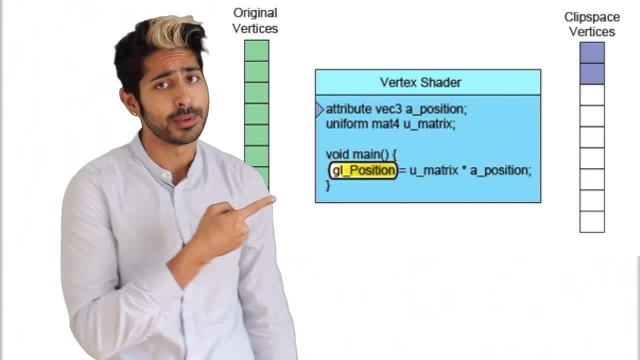 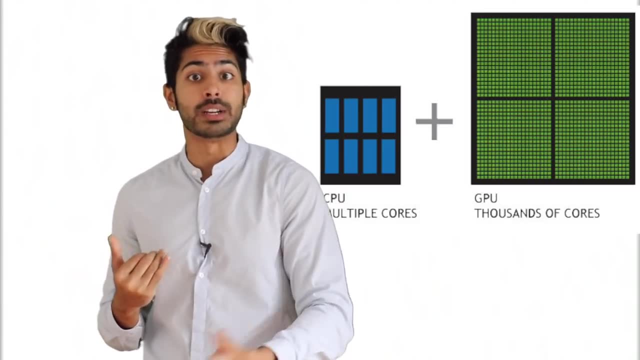 The coordinates are again transformed into camera space. These transformations require the use of matrix operations. For older games with simple models, this was entirely doable by a CPU. But as models got more complex, the amount of transformations outgrew the capabilities of a CPU alone. 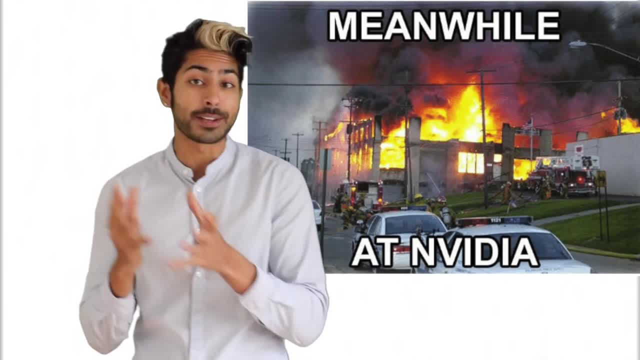 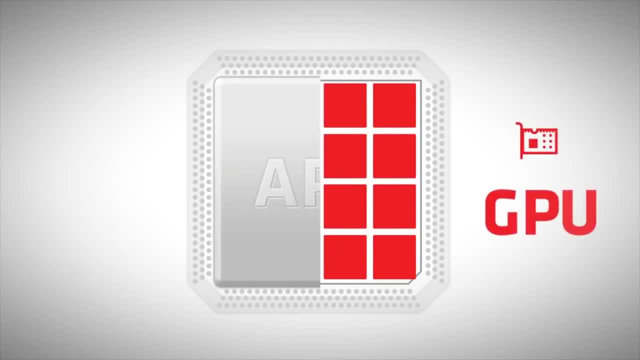 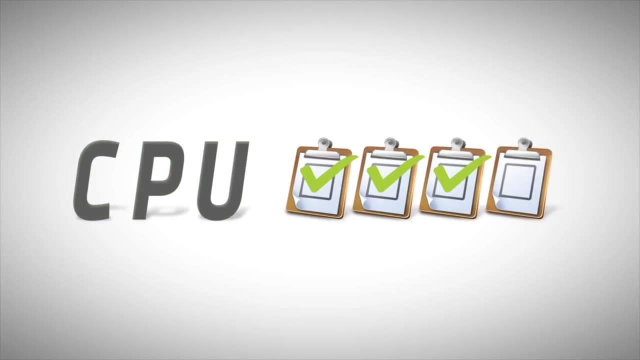 So a company named Nvidia came along and released the first graphics processing unit in 99,, capable of hardware transform and lighting. A CPU consists of a few cores optimized for sequential serial processing, while a GPU has a massively parallel architecture consisting of thousands of smaller, more efficient cores. 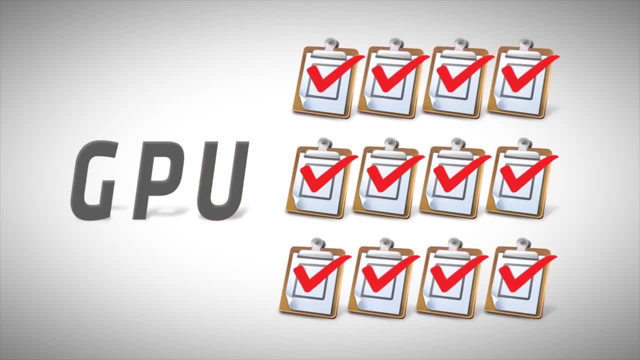 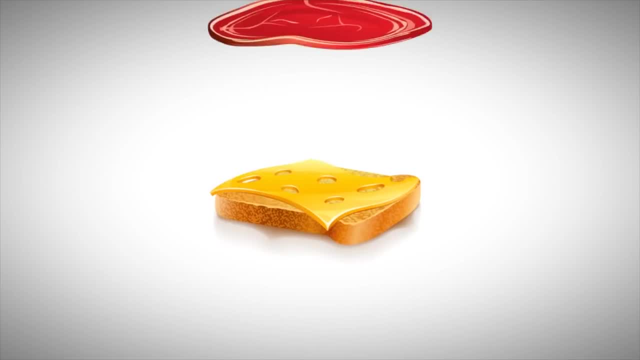 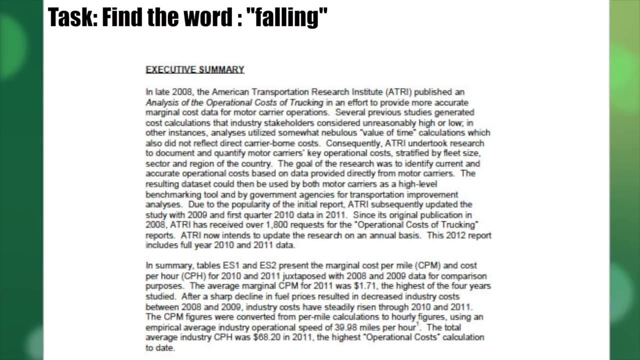 designed for handling multiple tasks simultaneously. So while traditionally software has been written for serial computation, where instructions are executed one after the other, there are some algorithms that can be framed to utilize parallel computation. Searching for a specific word In a document, for example, can be done serially. that means iterating through every word from. 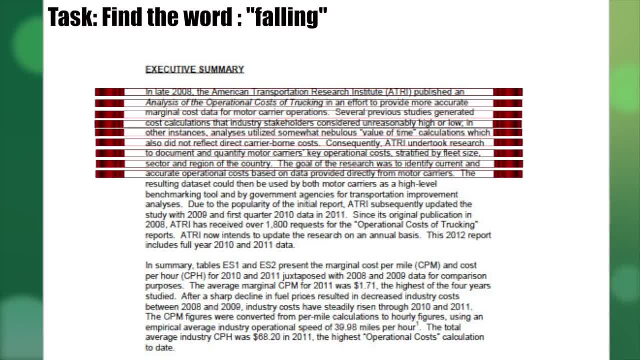 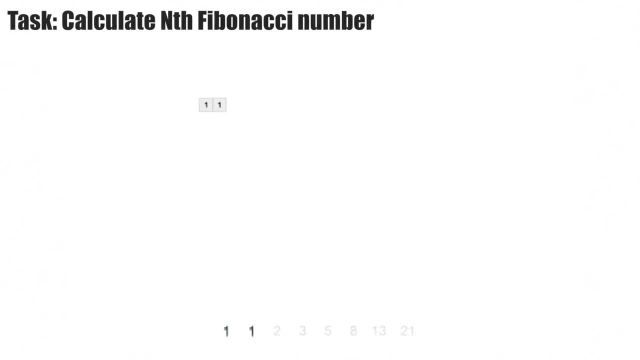 start to finish. but it can also be done in parallel by having 10 different workers search a different section of the document for our target word at the same time. But some algorithms, like calculating the nth Fibonacci number, can't be made parallel. 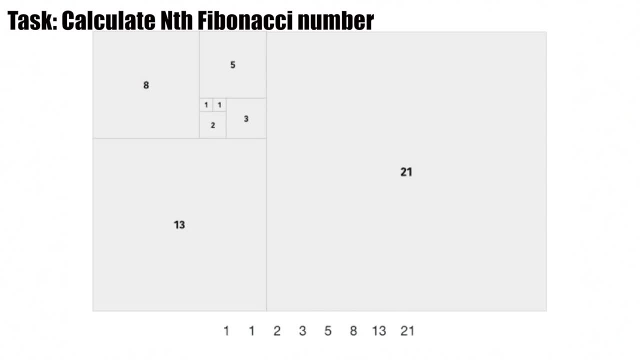 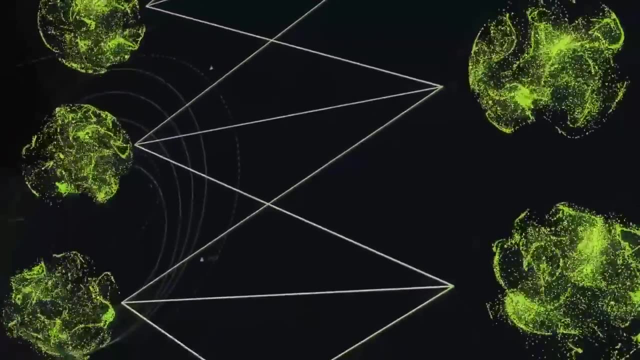 since we can only find it after the preceding two Fibonacci numbers have been calculated in order. Matrix operations for deep learning can easily be parallelized. Neural networks can have millions of parameters to train, all of which can be done much faster by utilizing GPUs. 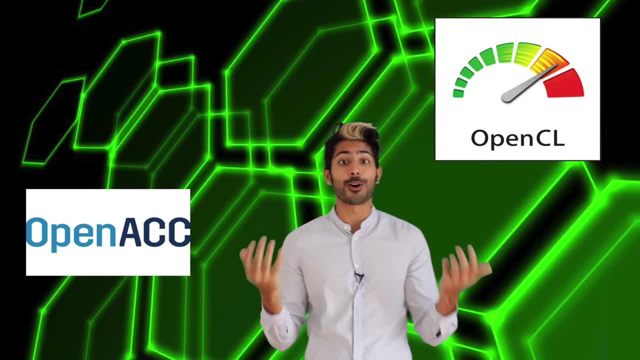 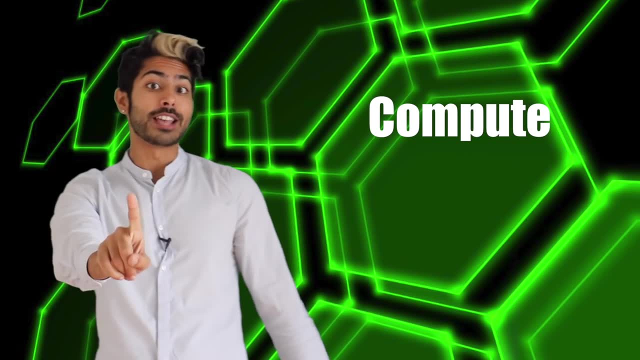 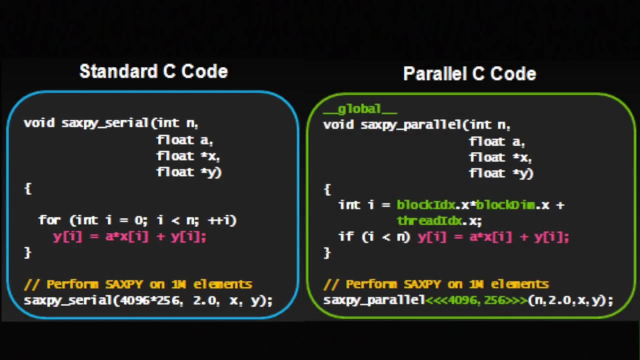 There are several programming frameworks out there that let programmers harness GPU cores, like OpenCL, OpenACC, but the most popular is NVIDIA's CUDA, which stands for Compute Unified Device Architecture. CUDA is a toolkit that acts as an extension of C, with its own programming model that lets 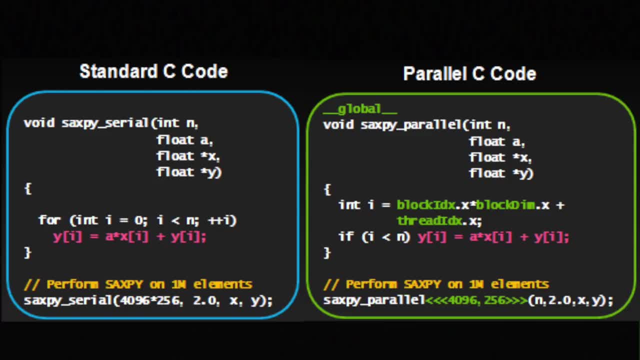 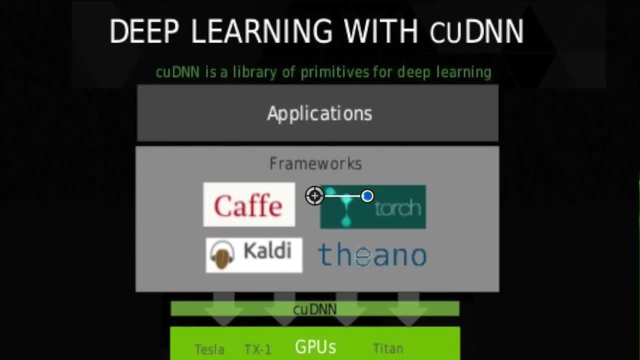 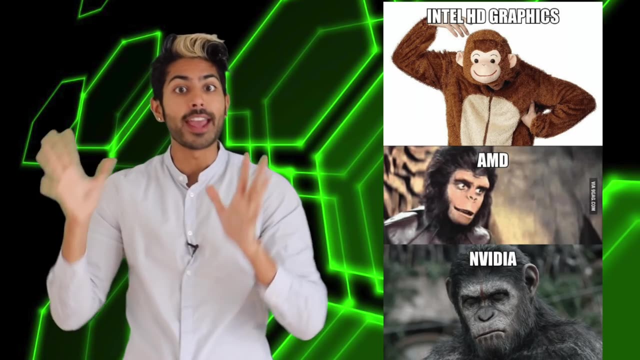 programmers run their code on NVIDIA's GPU. So let's get started. The CUDNN library, built on top of CUDA specifically for deep learning, is used by every single major framework, from TensorFlow to PyTorch under the hood. So let's talk about GPU architecture in the way that CUDA views it. 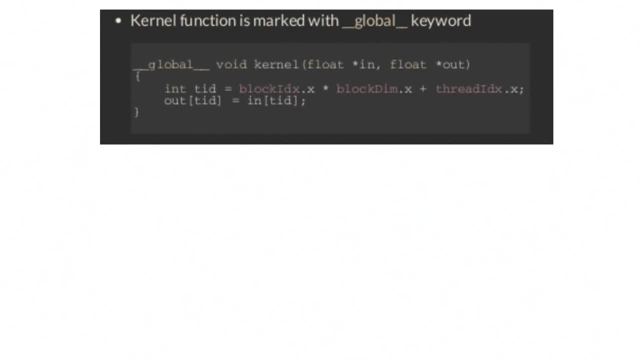 The key part of CUDA code is the kernel program. The kernel is a function that can be executed in parallel on the GPU. It's executed by an array of CUDA threads. All threads run the same code and each thread has an ID. It has an ID that it uses to compute memory addresses and make control decisions. 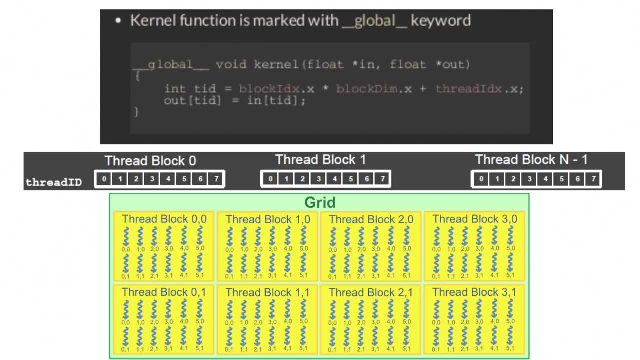 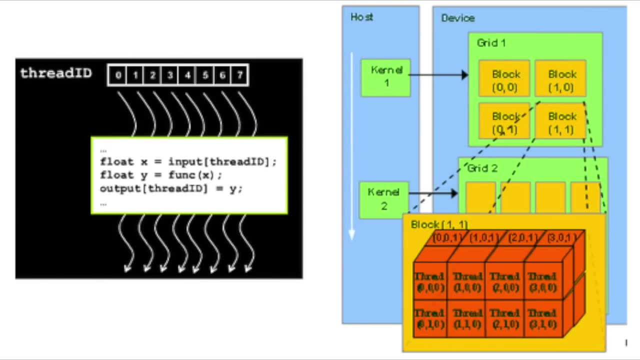 You can run thousands of these threads on the GPU, and CUDA organizes threads into a grid hierarchy of thread blocks. A grid is a set of thread blocks that can be processed on the device in parallel. Each thread block is a set of concurrent threads that can cooperate amongst themselves, and 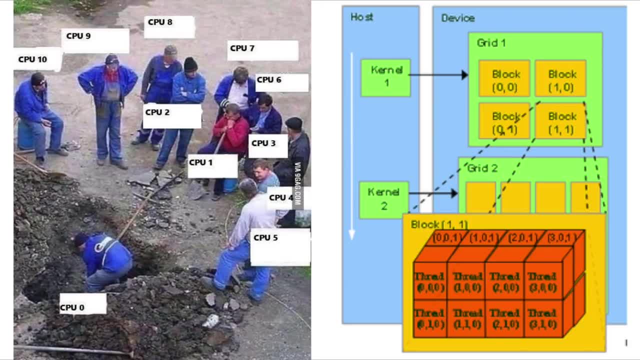 access a shared memory space private to the block. It's the programmer's job to specify the grid block organization on each kernel, Since it can be different each time, within the limits set by their specific GPU, Let's write some CUDA code to get a better understanding of how all these components 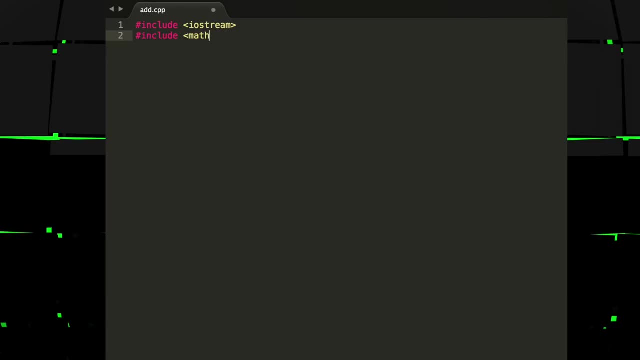 play together. We'll start with some basic C++. Our program will simply add the elements of two arrays with a million elements each. Only two dependencies: iostream, which will help us take input commands and show output results, and math, which defines various math operations we can use. 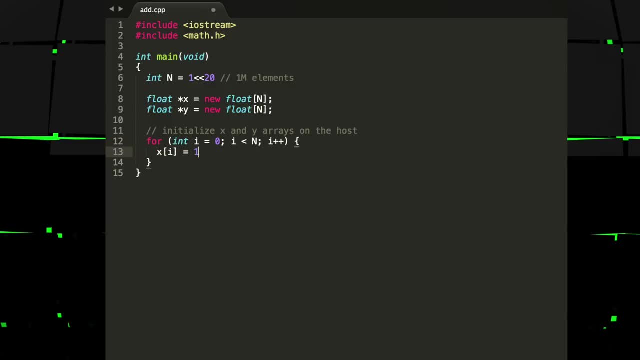 We'll initialize an integer array with space to store a million elements. Then we'll initialize pointers to both of our arrays x and y, with space allocated for both of them using our previously initialized variable n. We can fill both arrays by creating a for loop and filling each index in each array. 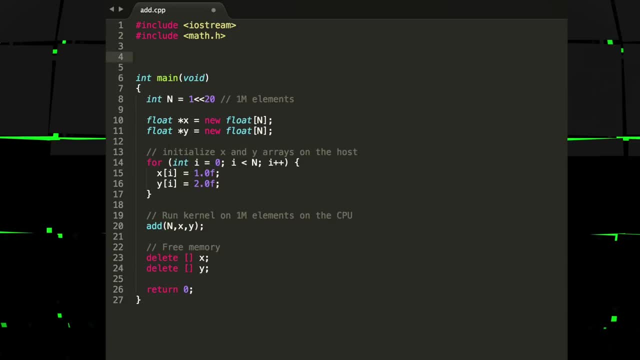 with float values, We'll use both filled arrays and the number of elements in each as parameters to an add function. In our add function we'll create a for loop to add all n elements into each array. For each array, we'll use the number of elements in each array to add parameters to an add function. 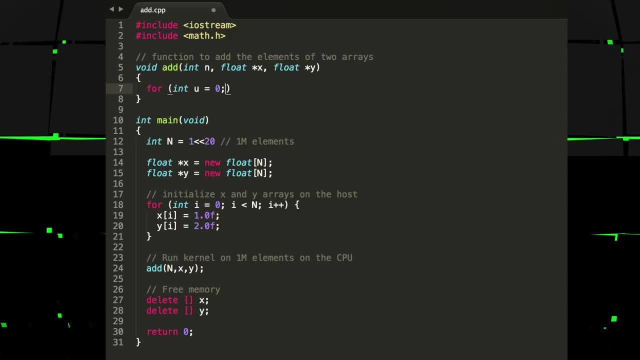 each array and set the result to each index in the Y array. After this loop is finished, Y will contain the sum of each element in both arrays. When we're done, we can free the memory from both arrays and exit the program by returning 0.. We. 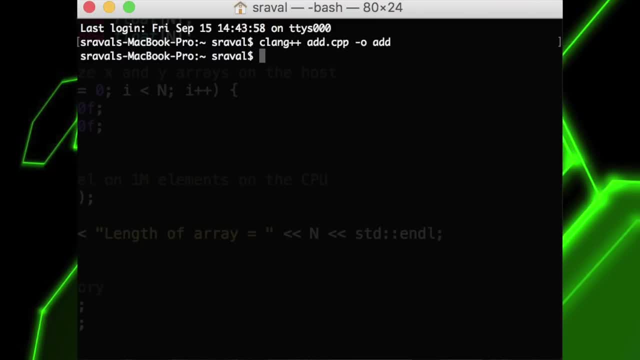 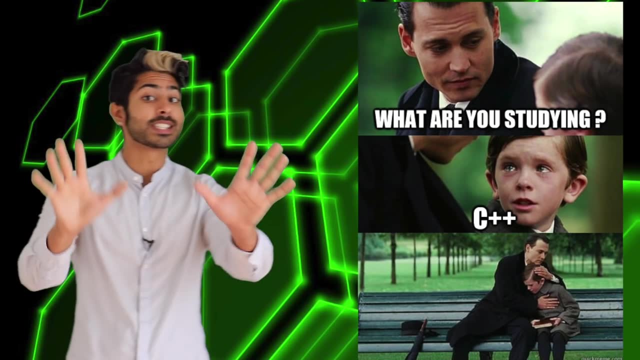 can save the code in this file as addcpp and compile it with a C++ compiler- Clang for me, since I'm on Mac G++ if you're on Windows or Linux. That was a simple C++ program, no CUDA needed, But adding the elements in both. 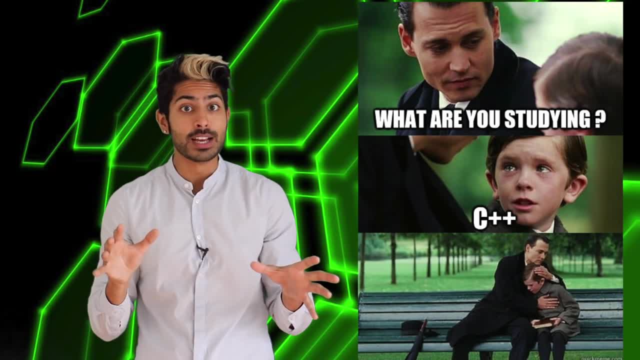 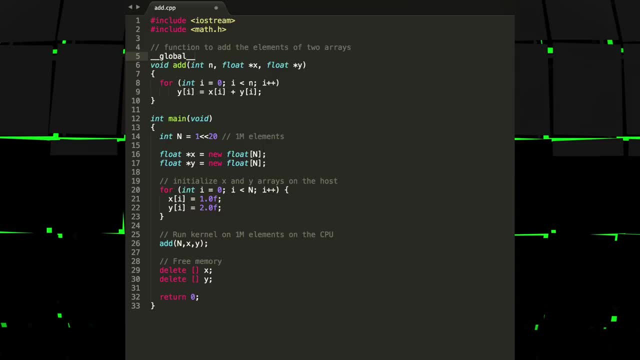 arrays can be parallelized on many cores of a GPU, So let's get turnt. The first step for us is to turn our add function into a function that the GPU can run, called a kernel in CUDA. All we have to do is add the global specifier. 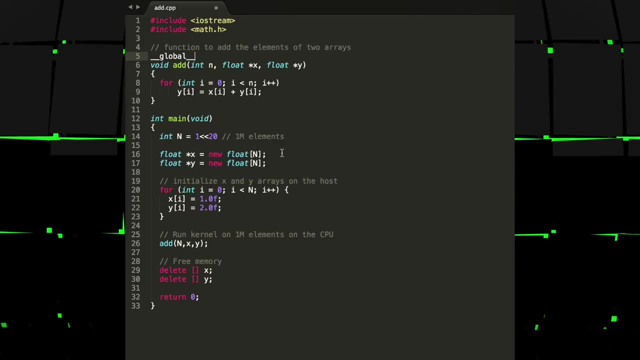 to the function and that'll tell the CUDA C++ compiler that this is a function that runs on the GPU and can be called from CPU code. We also need to allocate memory that is accessible by not just the CPU but the GPU as well. CUDA uses the concept of 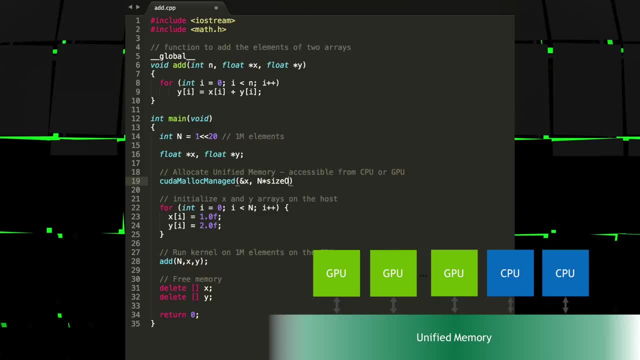 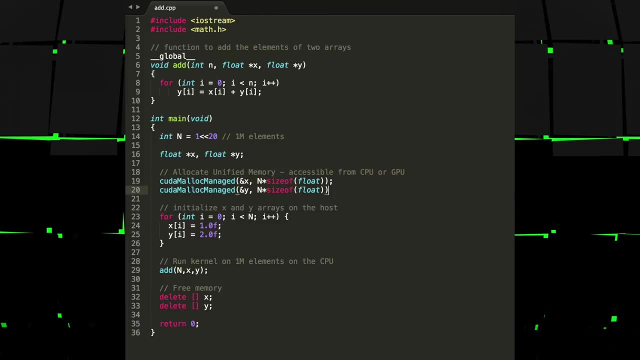 Y Unified memory. to make this easy, It provides a single memory space accessible by all GPUs and CPUs on your system. We'll need to replace the calls to new in our code with calls to CUDA, malloc, managed. This will allocate data in unified memory and returns a pointer that we can access from CPU or GPU code. 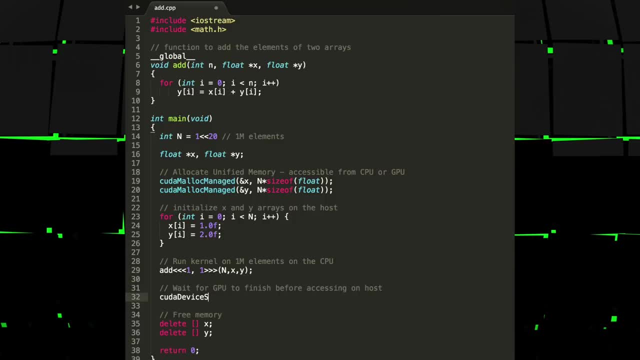 After this we can launch the add kernel on the GPU by using the triple angle bracket syntax. We'll just add it to the call to add before the parameter list and the CPU needs to wait until the kernel is done before it accesses the results because CUDA kernel launches. don't block the calling CPU thread. We 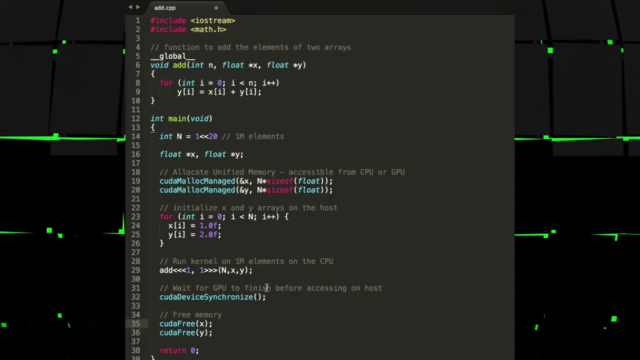 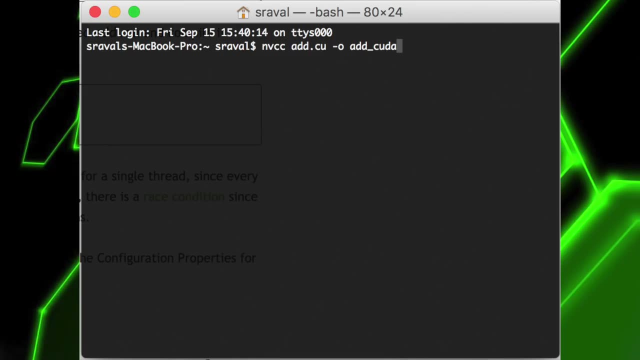 can make this happen by calling CUDA device synchronize before freeing the memory. Our one liner launched one GPU thread to run add. We can save this code in a file called addcu for CUDA and compile it with NVCC, the CUDA C++ compiler. As written, the kernel is only correct for a single thread, since every. 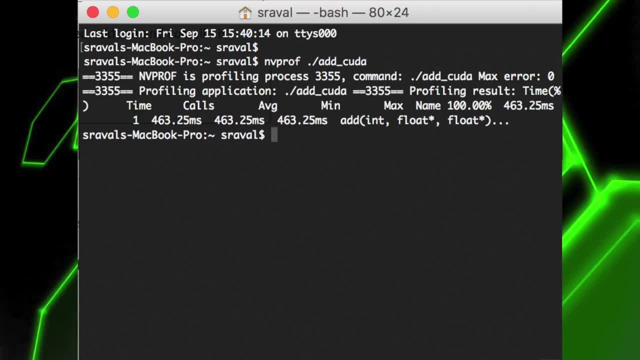 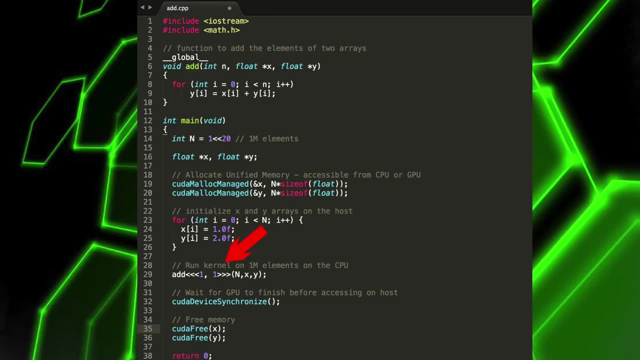 thread that it runs will perform. add on the whole array. We can find out how long it takes the kernel to run by using the GPU profiler as well. But can we make it faster? Our execution configuration tells the CUDA runtime how many parallel threads to use for the launch on the GPU. There are two parameters here. Let's: 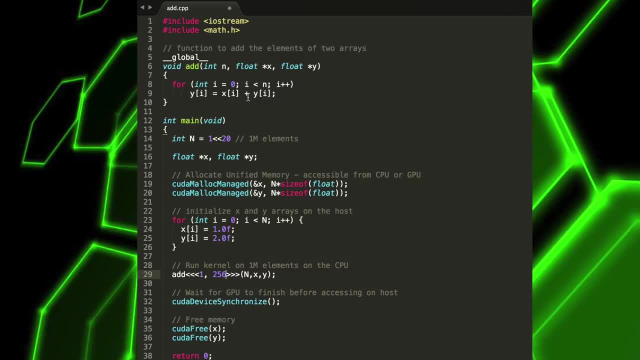 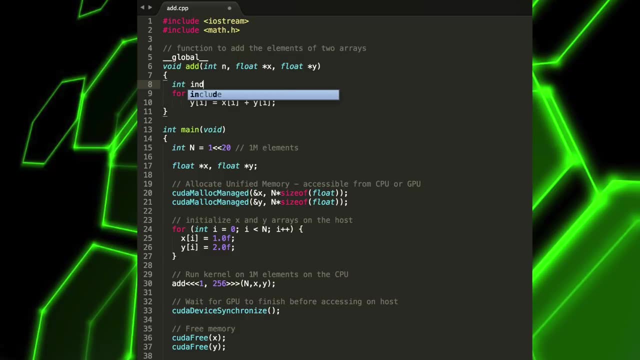 change the second one, which is the number of threads in a thread block. CUDA GPUs run kernels using blocks of threads that are a multiple of 32 in size, So let's try 256.. But doing this alone will cause it to do the computation once per. 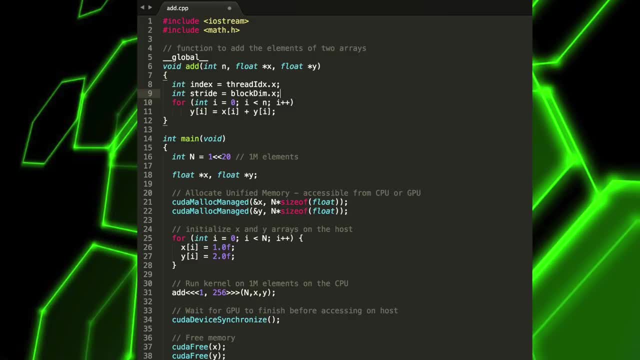 thread Rather than spreading the computation across parallel threads. To do it properly we need to modify the kernel. We can get the indices of the running threads using the thread ID keyword for the current thread in its block and the block dim keyword for the number of threads in the block. We can 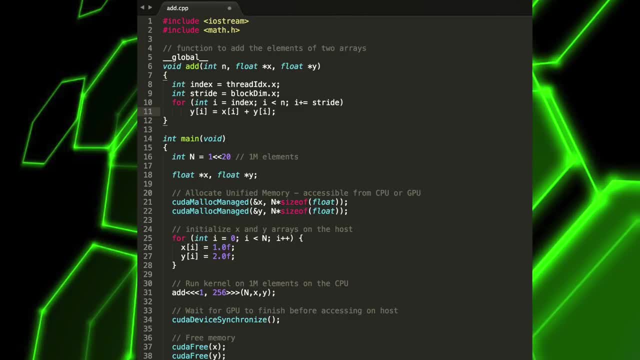 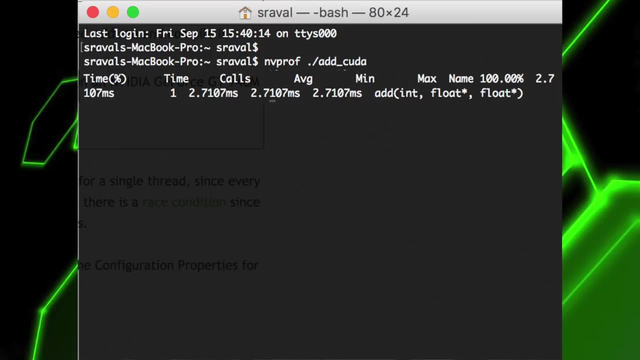 modify the loop to stride through the array with parallel threads. If we save it and run it again, we'll see a huge speedup from using one thread to 256 threads. so this makes sense. To summarize what we've learned, CUDA is a toolkit that lets programmers use NVIDIA's 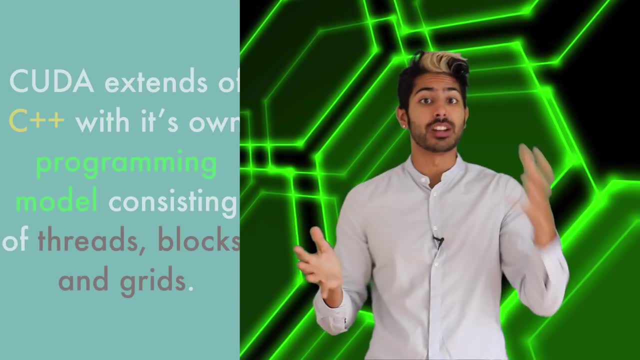 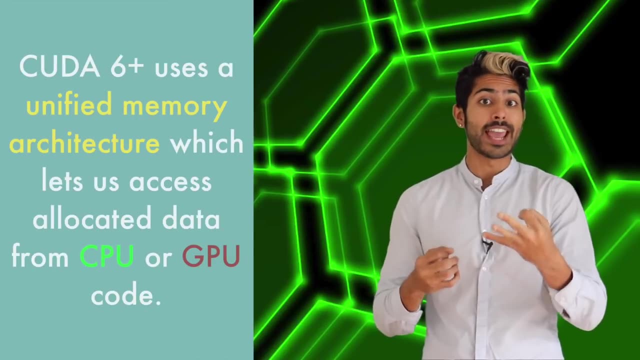 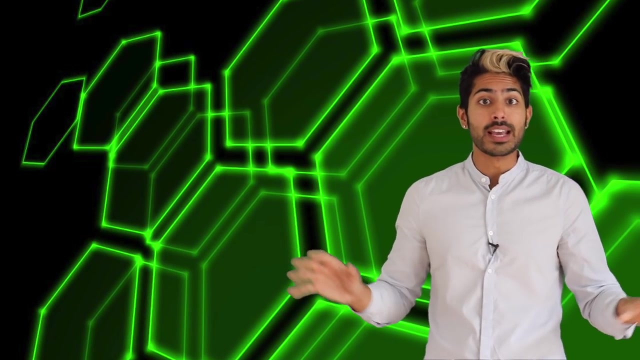 GPUs to parallelize their code. It's an extension of C, with its own programming model consisting of threads, blocks and grids, And the newer version uses a unified memory architecture which lets us access allocated data from CPU and GPU code. The winner of last week's coding challenge is Alberto Garcés. 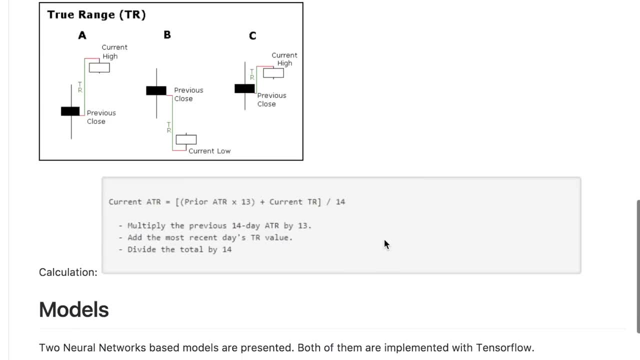 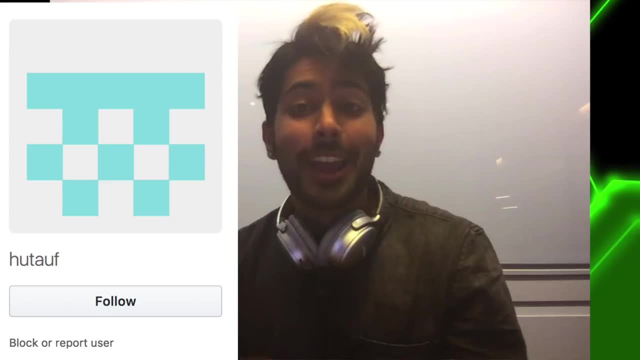 He used two neural network-based models that he implemented in TensorFlow, with popular indicators from the field of market analysis, to predict trends. Give his code a star on GitHub. And the runner-up is Kutauf, who converted stock prices into audio data and ran DeepMind's. 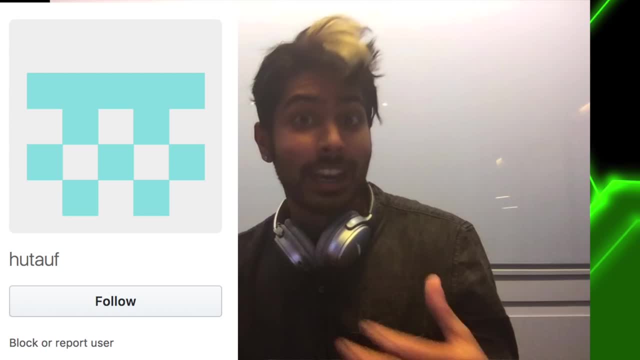 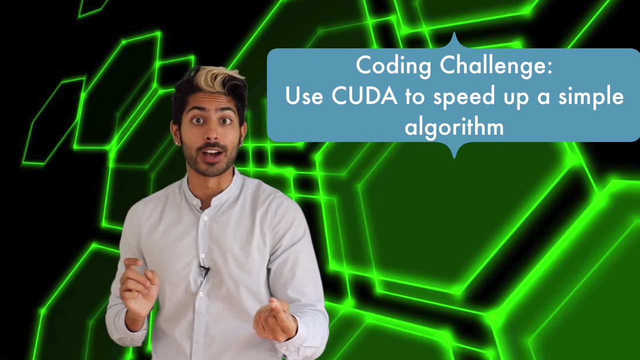 WaveNet on it. What a wild and brilliant idea. I love it. This week's challenge is to add CUDA to a simple algorithm and benchmark just how fast the CPU and GPU work. Details are in the readme. post your GitHub link in the comments and winners will be.